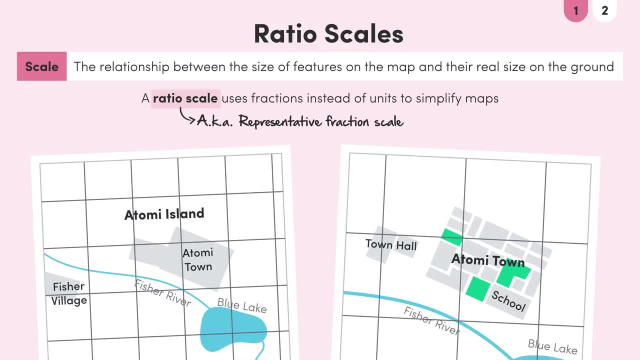 Let's look at two maps of Atami Island. We can see the 1 to 50,000 scale on the first map and the 1 to 25,000 scale on the second map. Let's think about why these different scales are handy If you are going out for a walk. 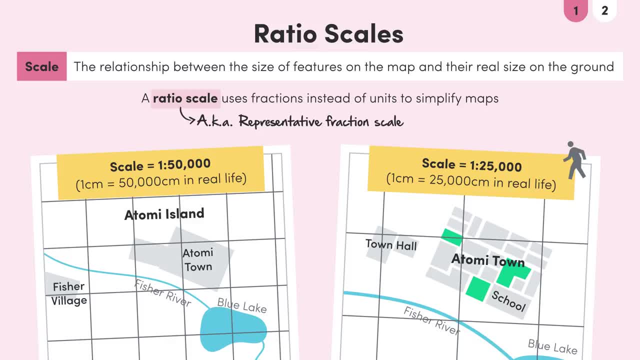 around Atami town. you may want a scale of 1 to 25,000, meaning that 1 centimetre on the map is 25,000 centimetres or 0.25 kilometres in real life For a cycle ride around Atami. 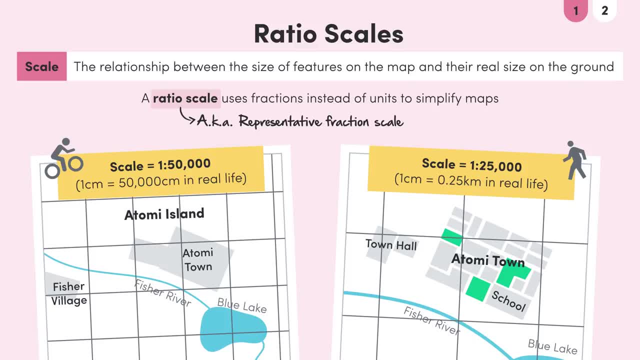 Island, though you'll be travelling further and faster, so a scale of 1 to 50,000 may be more appropriate. Let's look at the second map, where 1 centimetre on the map is 50,000 centimetres or 0.5 kilometres. 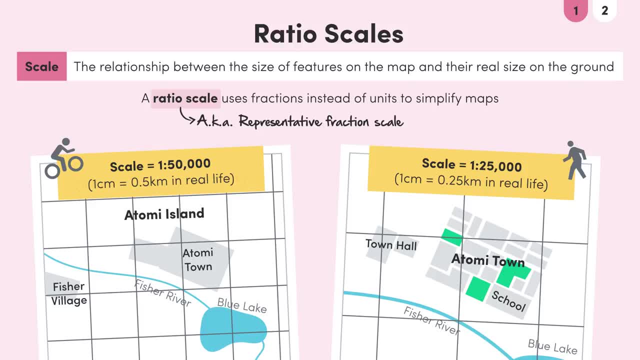 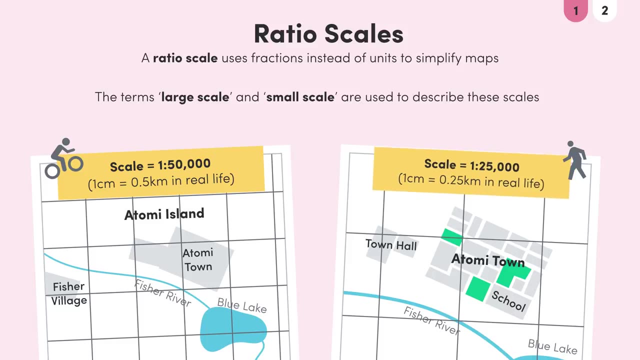 in real life. This is just because you can travel further on the second map without having to move it or turn it over. The terms large scale and small scale are used to describe these different scales. However, they can be confusing. You might think that the second 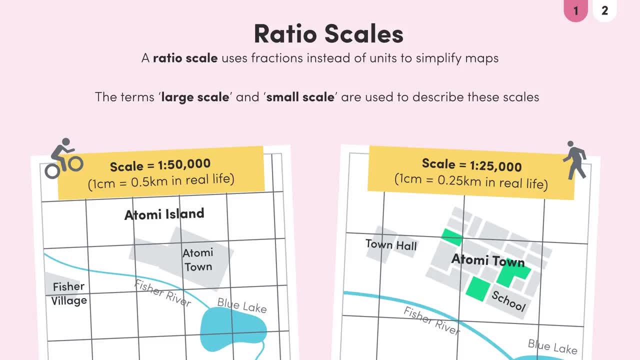 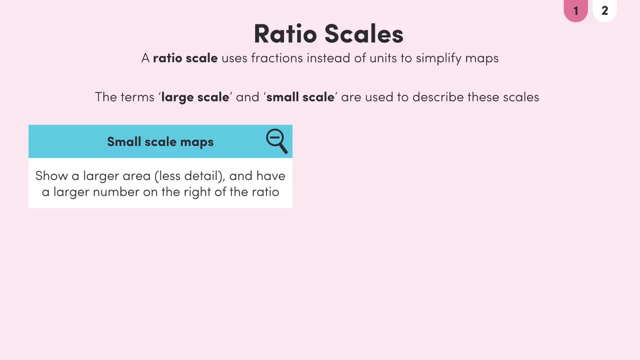 map with a 1 to 25,000 scale is the small scale map, but actually it's the opposite. Small scale maps show a larger area or less detail, meaning that the number to the right of the ratio is much larger, such as 1 to 250,000.. Large scale maps show more detail. 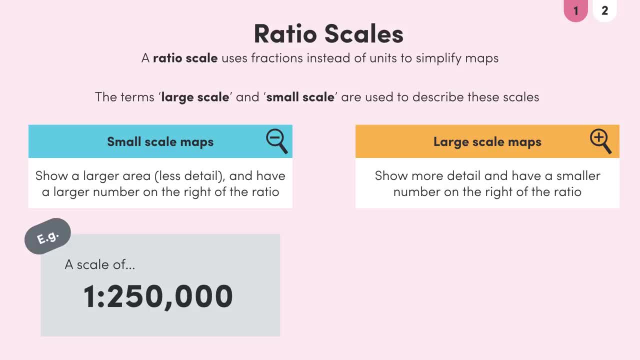 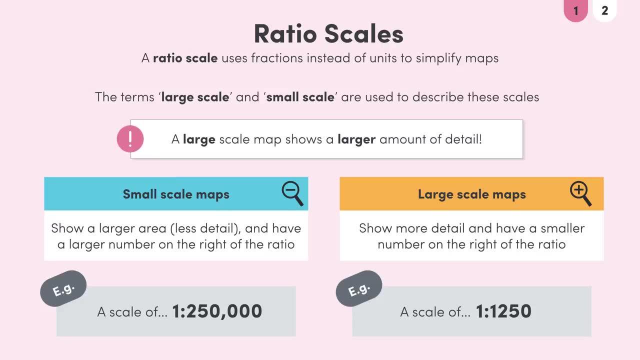 and so the number on the right of the ratio is smaller, such as 1 to 1,250.. I like to remember this by. a large scale map shows a larger amount of detail, So deciding what scale to use for cartography is really important. 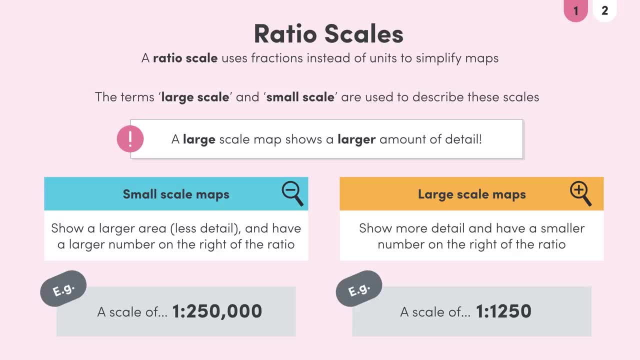 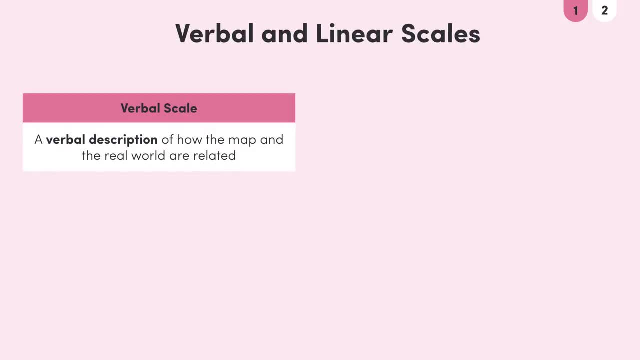 If the scale is too large, you'll have to keep moving the map Too small and the map may not show enough detail. There are also verbal and linear scales which can be used in mapping. A verbal scale is simply a verbal description of how the map and real world are related. For example, 1. 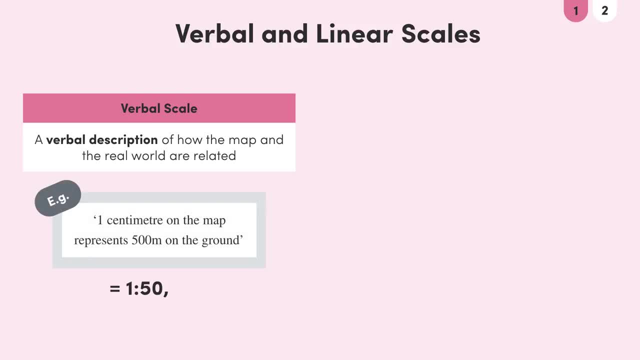 centimetre on the map represents 500 metres on the ground is a simple verbal scale which translates to 1 to 50,000 in ratio scale. Linear scales are the sort of scales that you can see on many maps that you find in textbooks and on the internet. These scales visually show how much distance is represented. 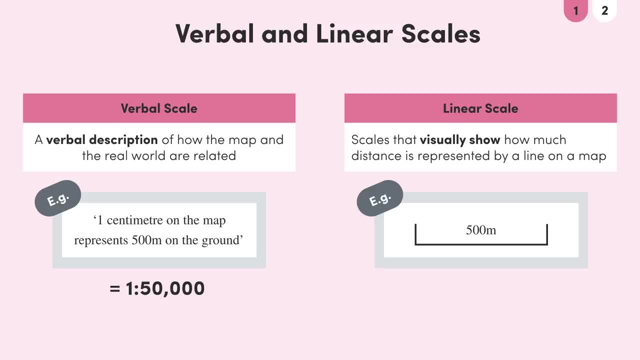 by a certain line on a map. Taking the stated distance, say 500 metres, and dividing it by the length of the line, say 2 centimetres, gives us the ratio scale once more. In this case that's 1 to 25,000.. So scales are most commonly represented in maps as ratios. but 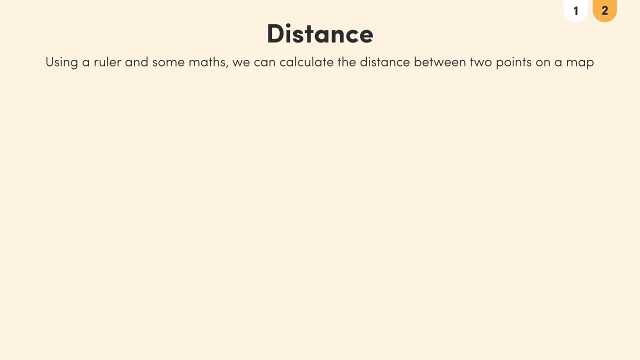 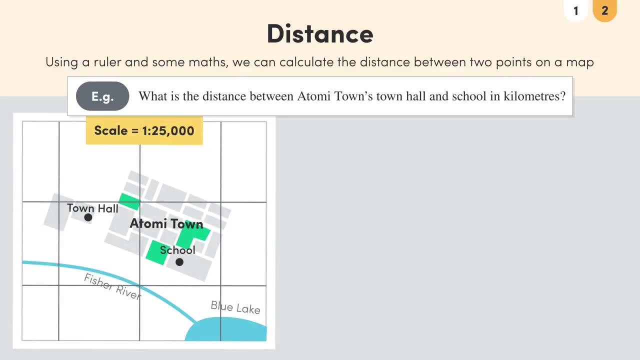 how can these be used to calculate distances between two points on a map? The easiest way to do this is simply with a ruler and a little maths. Firstly, line up the ruler between the two points, ensuring that zero on the ruler is at one point, and. 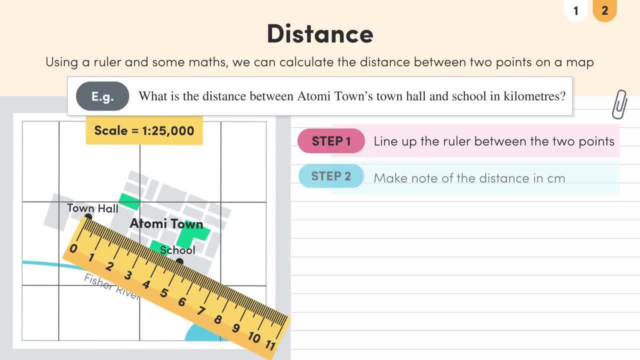 the ruler cuts straight through each point. Then make a note of the distance in centimetres between them. Next, compare this measured distance to the ratio scale. For example, if the distance between the points on the map is 0,, then the distance between the points on the map is: 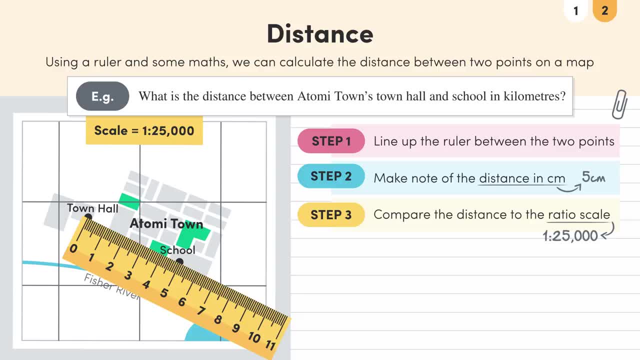 5 centimetres and the scale of the map is 1 to 25,000,. you can times the length you measured by the scale to get the distance in real life. So 5 centimetres times 25,000 is 125,000 centimetres. 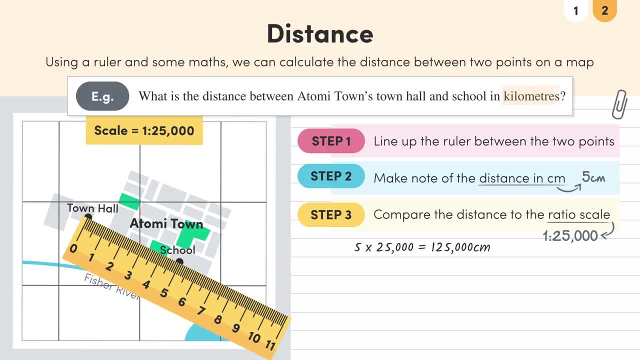 In your exam, though, you'll have to give an appropriate unit, for example kilometres. To convert 125,000 centimetres to kilometres, you'll need to divide by the number of centimetres in a kilometre. So, in kilometres, the distance is 125,000 divided by 100,000, which equals 1.25 kilometres. 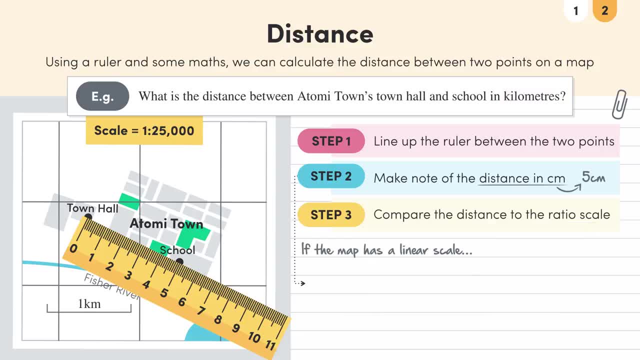 As an easier solution, if the map has a linear scale, which may be found towards the bottom of the map, you can compare your measured distance to this scale too. To do this, move your ruler with the measured distance to the scale at the bottom of the. 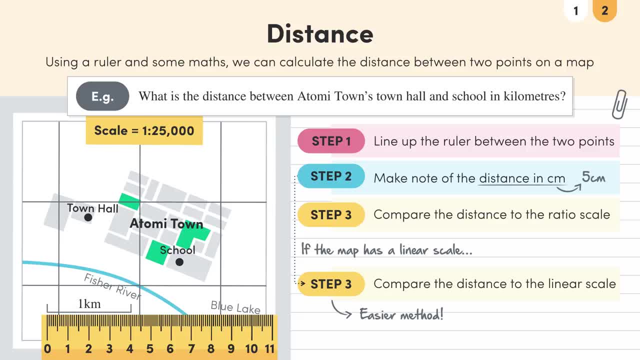 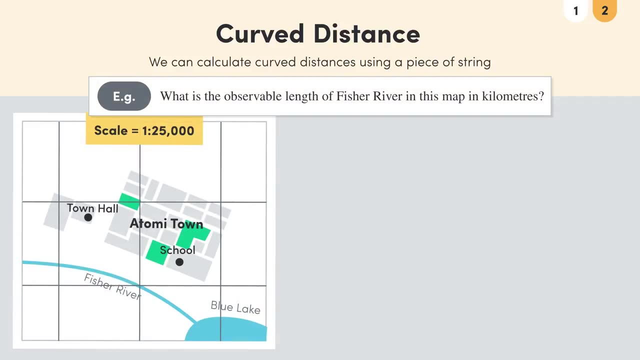 map and use the scale to read the distance between the points. Once again, make sure that the zero on your ruler lines up with the scale. Sometimes, though, you may need to measure a distance that is not straight but curved. In this case, a piece of string can be used. First, we need to measure the distance on 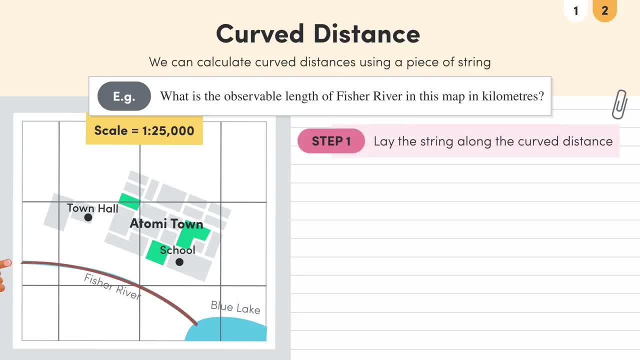 the map by carefully laying the string along the curved distance, making sure to keep hold of the zero point. Then, when stretched back out, the string can be compared to your ruler and measured using the same method of multiplying by the scale. The important thing to remember.